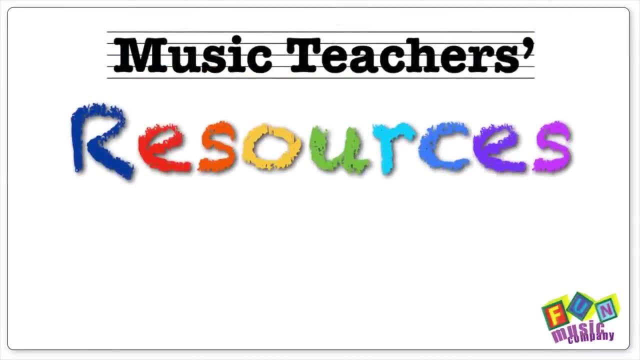 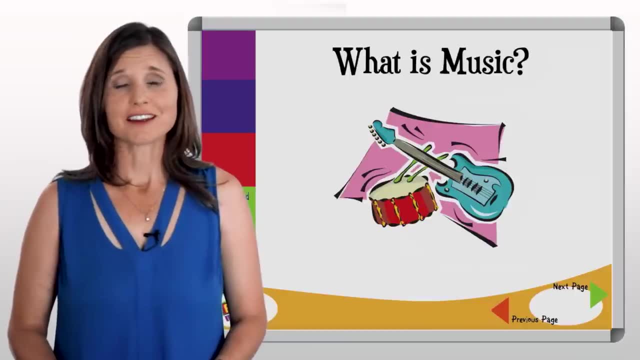 Hi, it's Janice Tuck here, and today I wanted to share with you some free ideas for primary or elementary school music lessons. Now I know, particularly at the early levels, we need to be getting children's minds switched on right from the word go. Therefore, we need 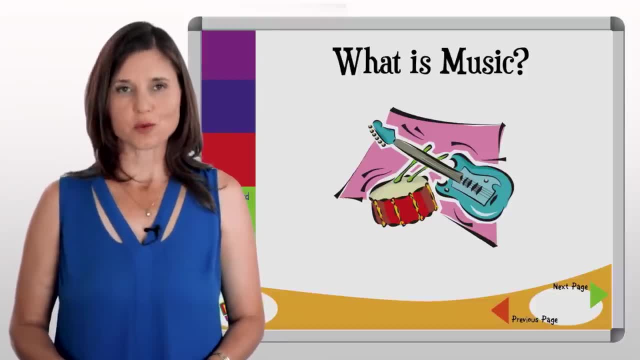 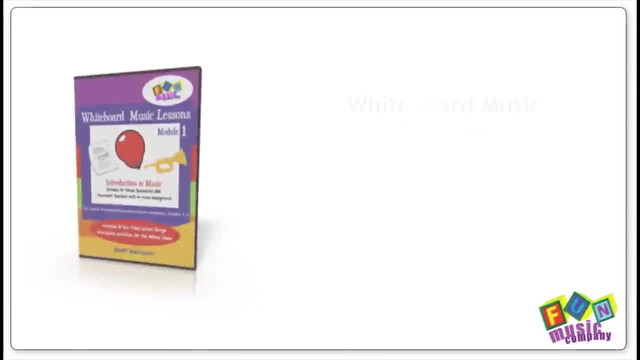 some ideas that really get things moving right away. So for this reason, today I thought I'd share a really simple concept with you, which comes from our very first lesson on the introduction to music module. It starts from the premise that we begin where the children are and we 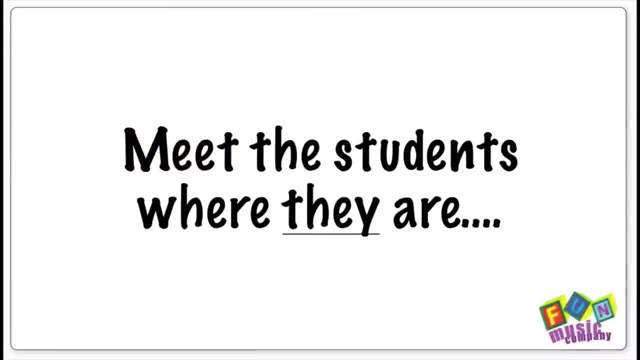 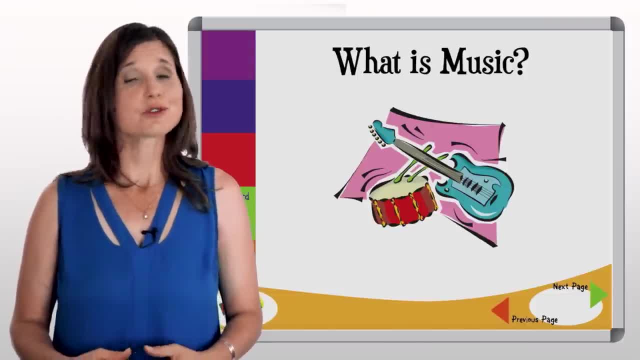 find out what music means to them. All children will have different ideas about this Now. some will have been to preschool music or dance classes since they were two or three years old, and some, who might have had parents who are really into music, might listen to. 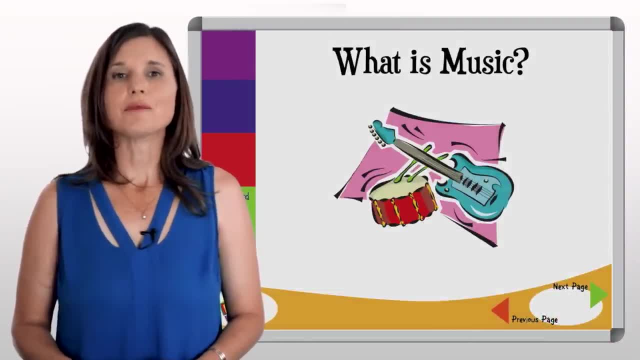 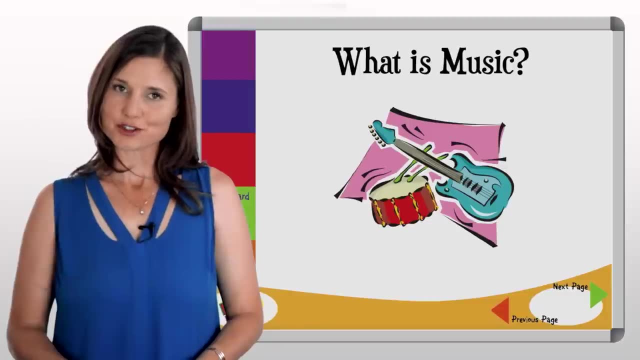 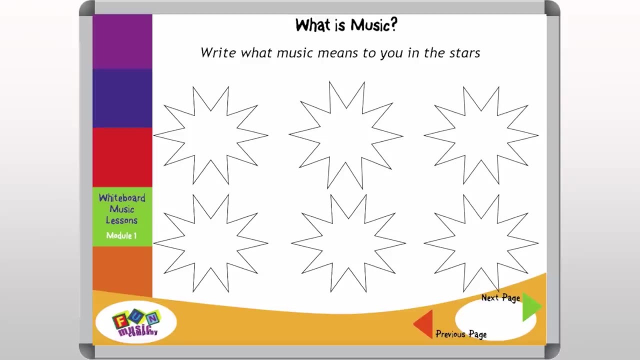 bands and go to concerts all the time. Some, however, might never have listened to music other than by accident. So it's important that we find out when we're first meeting these children for the first time. So that's why I've got a few whiteboard slides to share with you to start discussion with today, One where 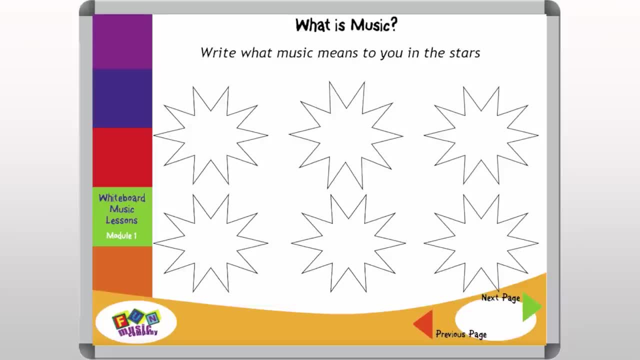 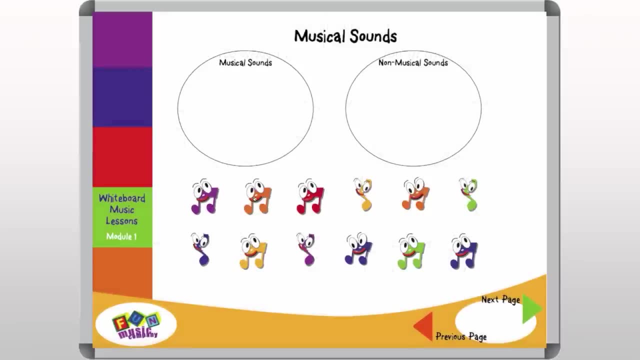 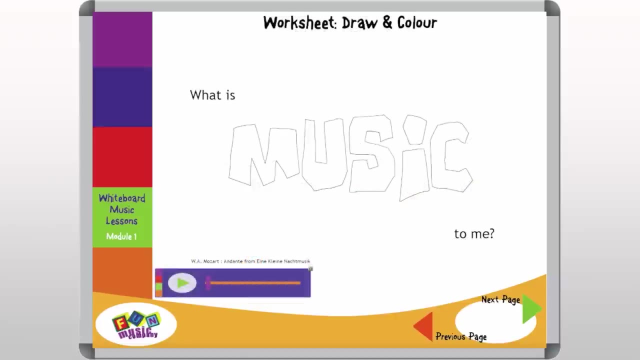 they'll just write what music means to them by writing in the stars, One where they'll listen to a variety of different sounds and discuss which ones are musical to them, And then the worksheet where they'll draw freely what music means to them. I think you'll find this a most insightful. 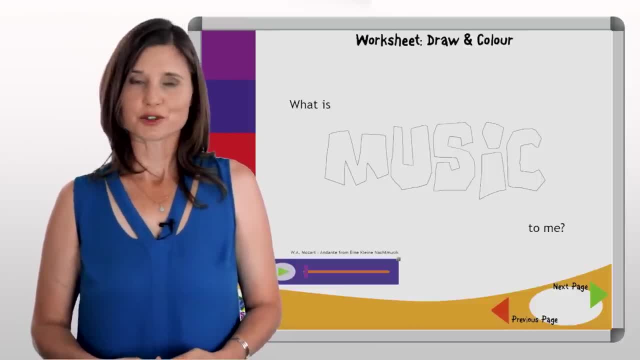 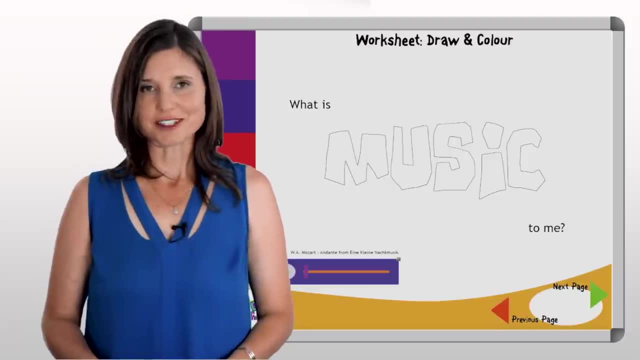 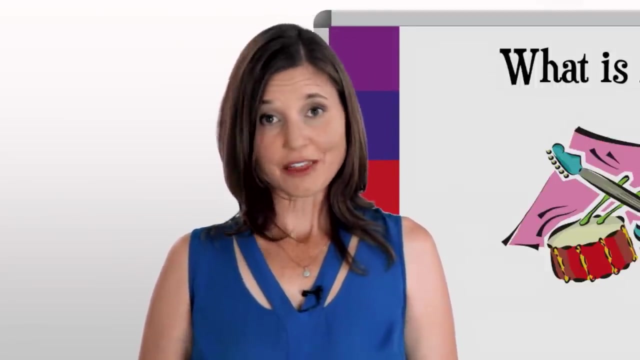 lesson and you'll get some fascinating responses back from the children and you'll be able to move on from there with increasing and expanding their awareness of music. So, as always, let me know how you get on and I will see you next week with another free resource. 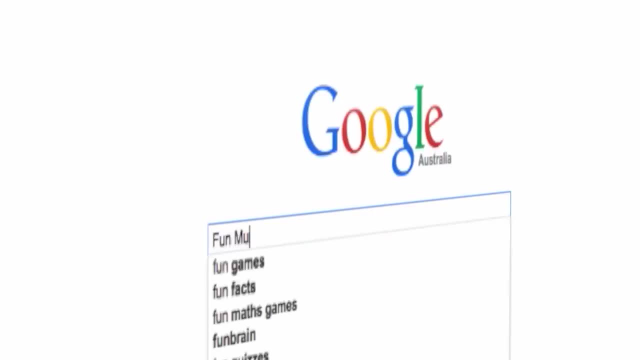 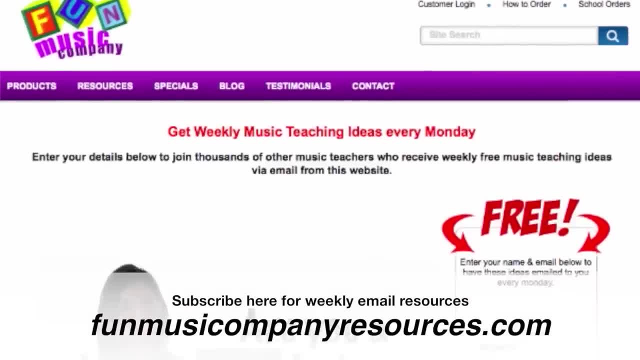 our weekly emails. We'll make sure you're subscribed to our weekly emails. We'll make sure you do head over to funmusiccompanyresourcescom, because I will make sure that you get an email each and every single week and be some of the first people to see it.